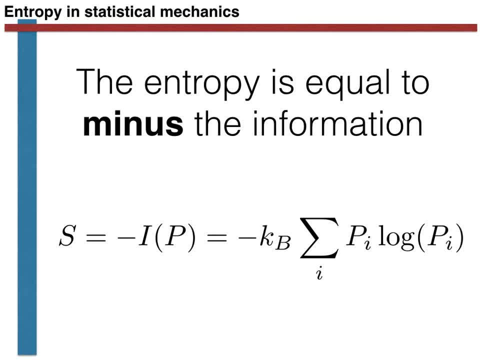 In statistical mechanics, we set the entropy equal to minus the information, as shown here. Let's consider what this means for a system that has a uniform probability of being in one of w different microstates. first, As the distribution is uniform. As the distribution is uniform, 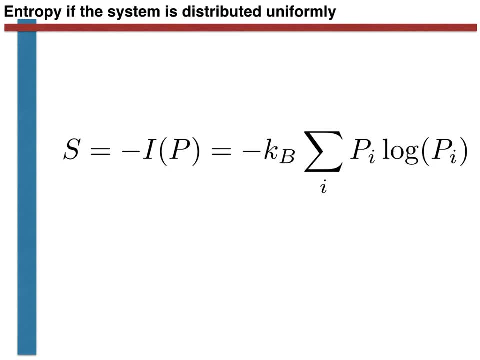 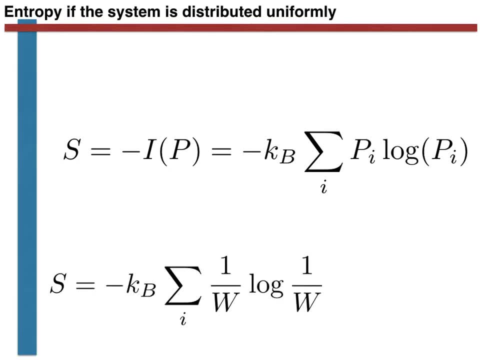 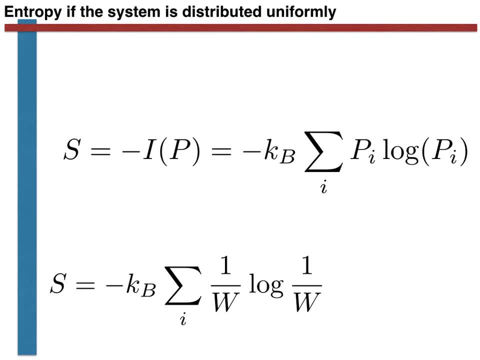 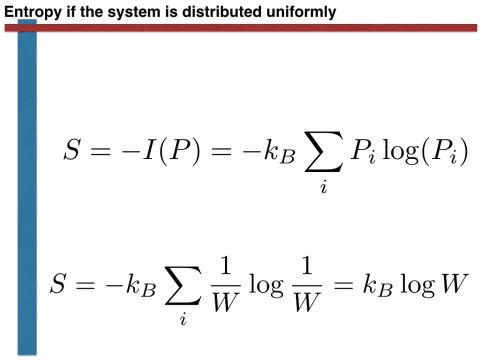 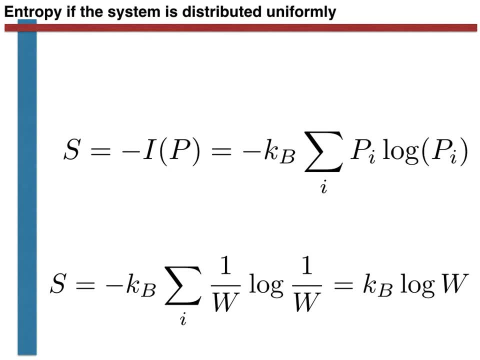 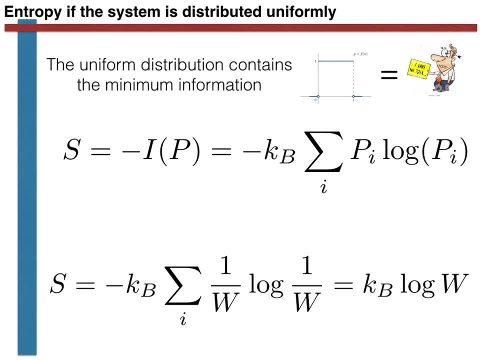 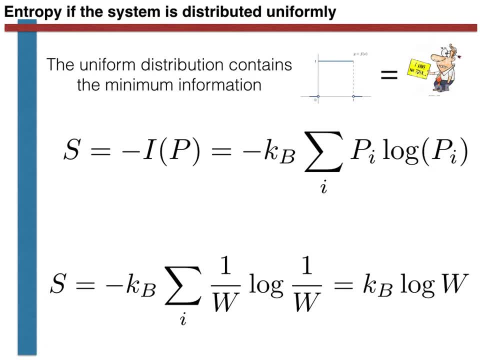 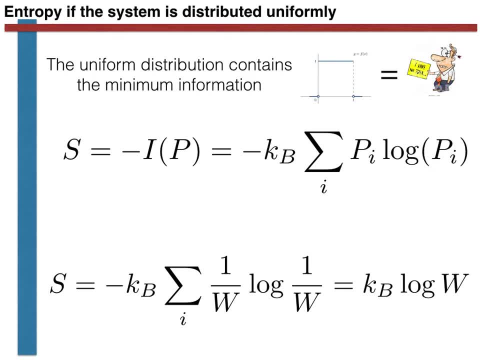 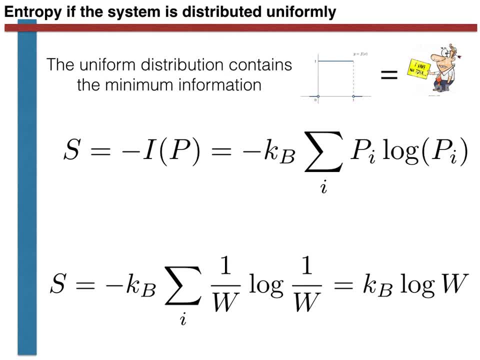 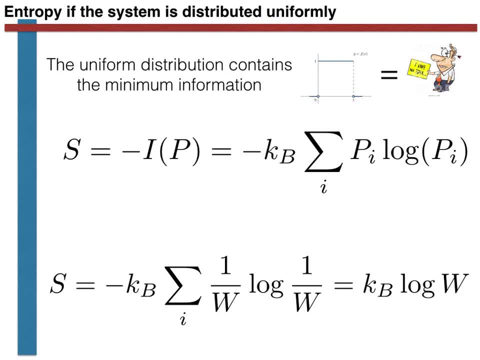 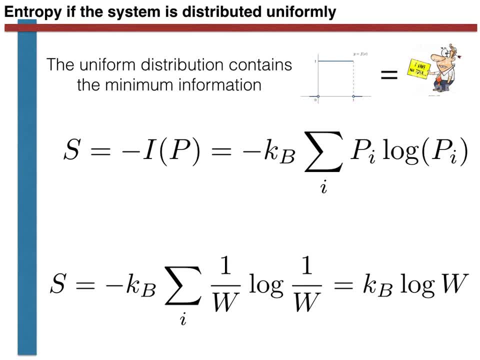 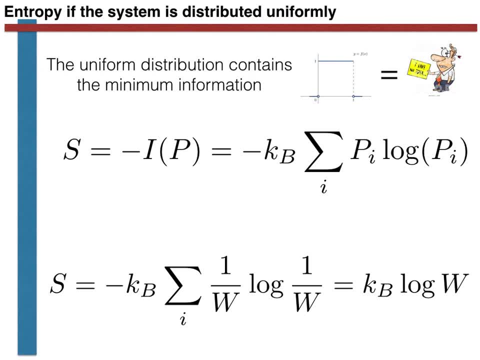 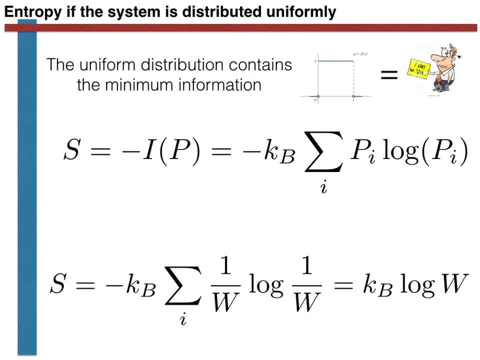 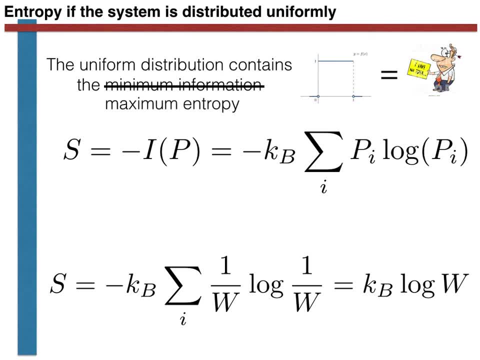 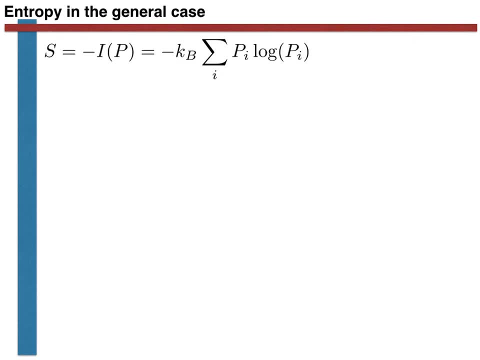 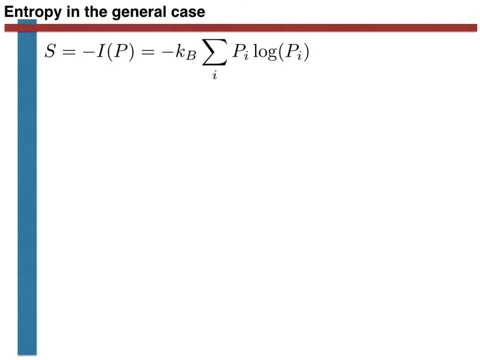 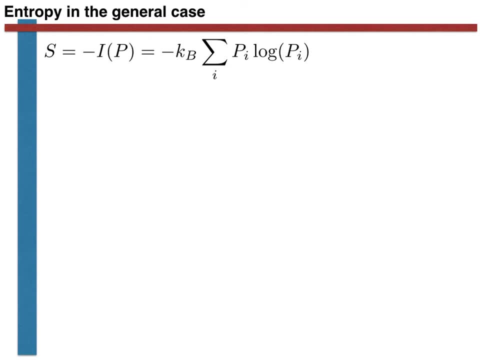 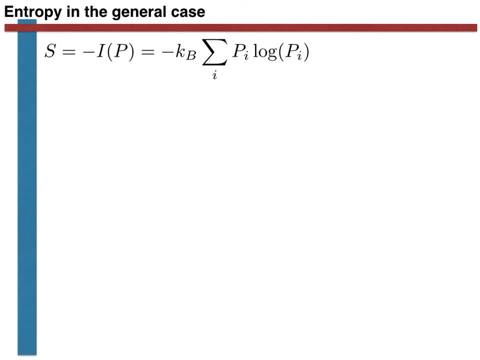 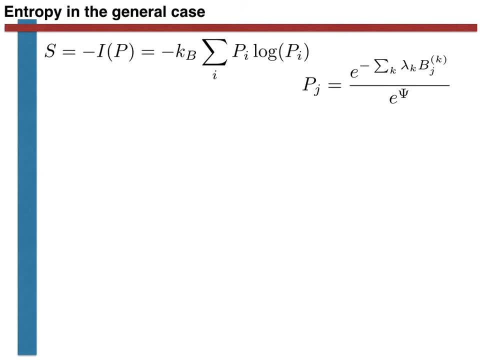 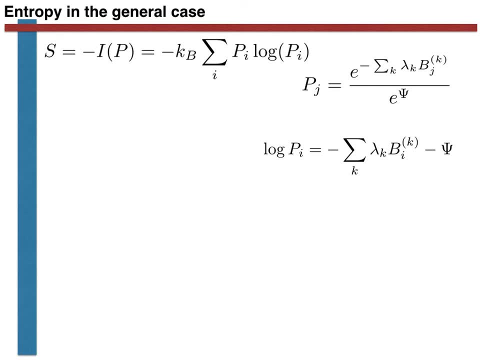 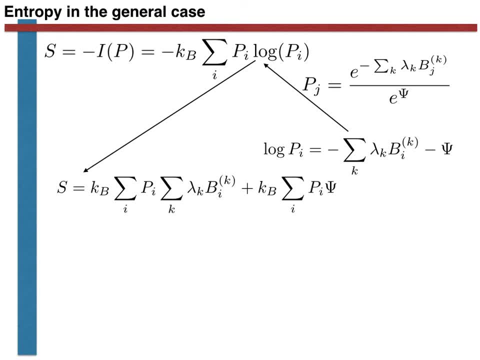 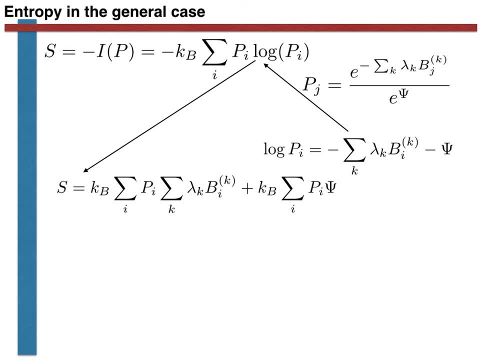 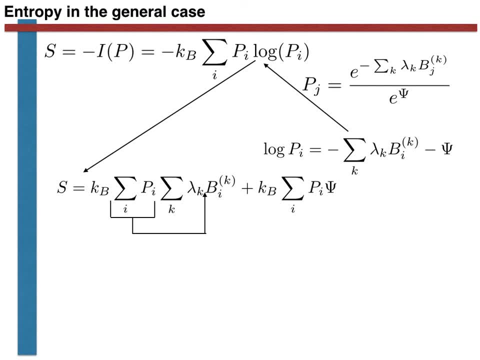 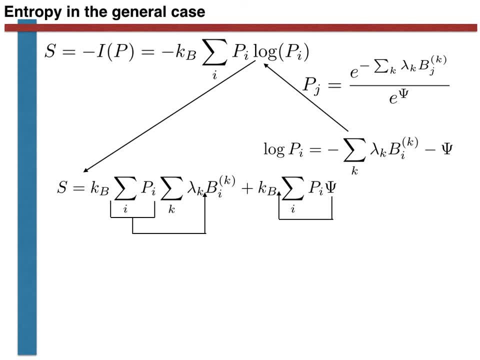 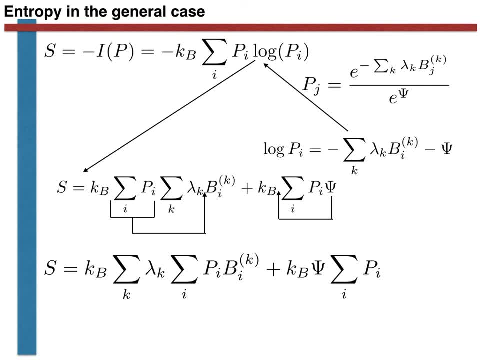 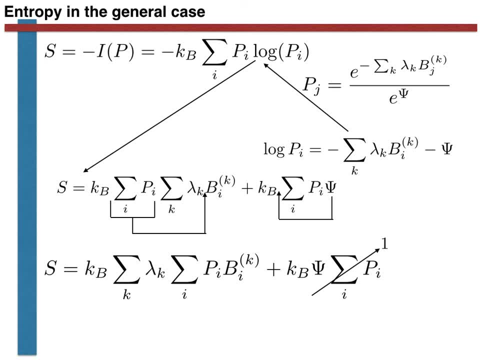 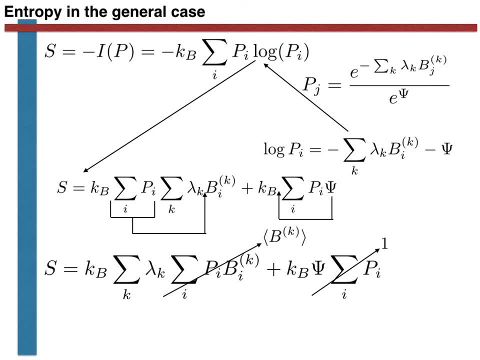 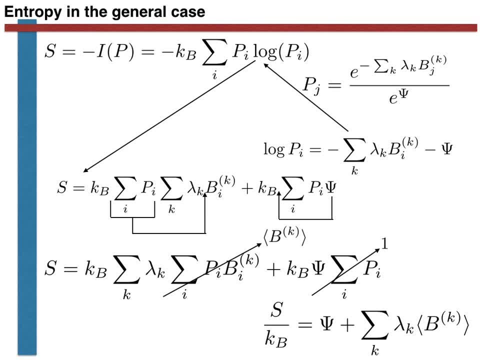 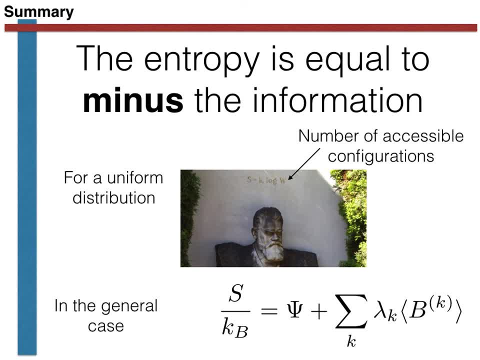 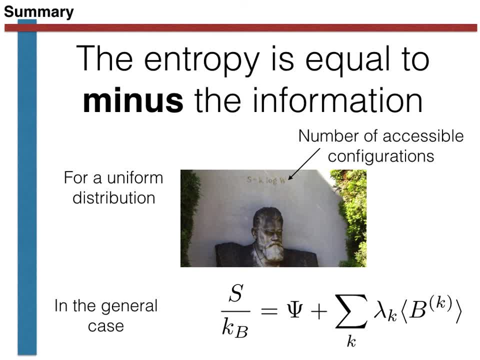 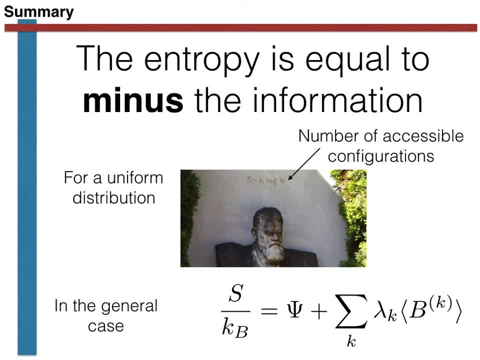